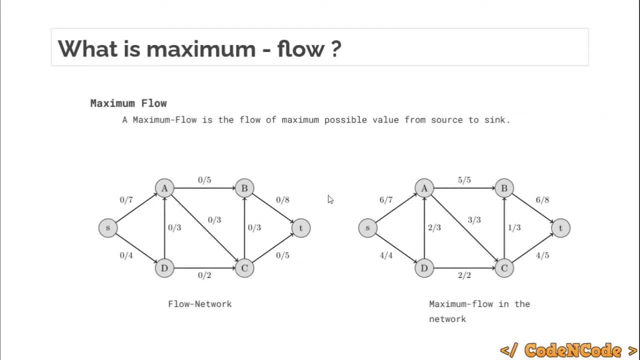 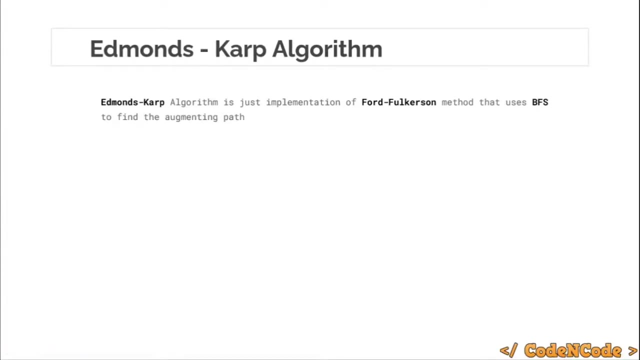 have to find, we need to devise an algorithm which can enable us to find the maximum possible flow through source to the terminating point or from source to the sink. for that we have already seen for Fulkerson method. but the problem with for Fulkerson method is that 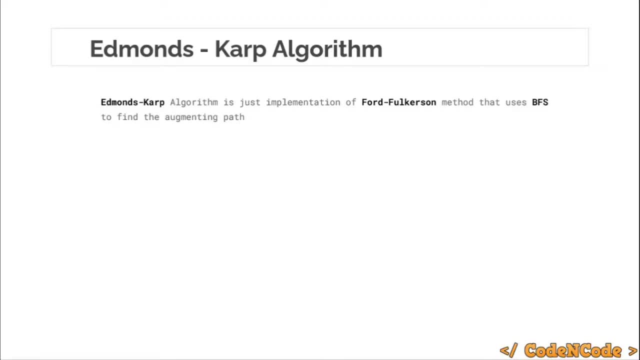 it does not specify how to find the augmenting path, while Edmund Scarp's algorithm is just an implementation of Fulkerson algorithm and that uses BFS to find the augmenting path. so it also specifies how to find the augmenting path, while for Fulkerson algorithm does not. now the time complexity of Edmund Scarp. 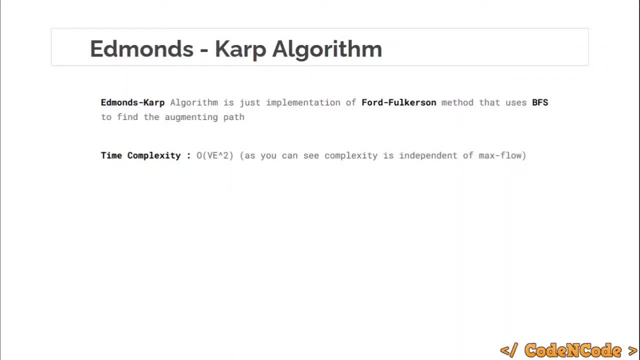 algorithm is VE square, where V represents the vertex set and E represents the edge set. now, as you can clearly see, the time complexity in the worst case is independent of max flow, while for uh, for the Ford Fulkerson method, the time complexity was dependent upon maximum flow. 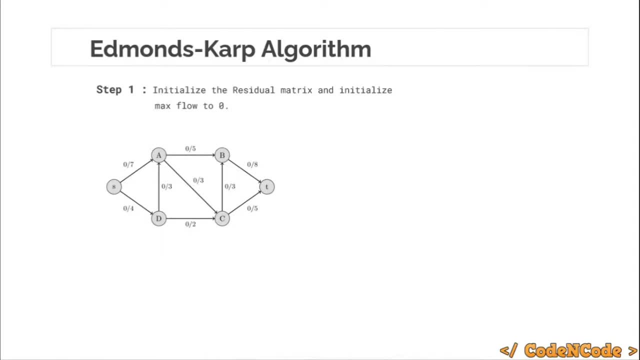 now, uh, Edmund Scarp algorithm is actually, uh, I think, two-step process that I played: first, initializing the residual, residual capacity matrix and see, as you can see here, this: each cell, of course, represents this. this cell represents SA, so this will represent the capacity of the edge as a this edge. similarly, this cell would represent AB. 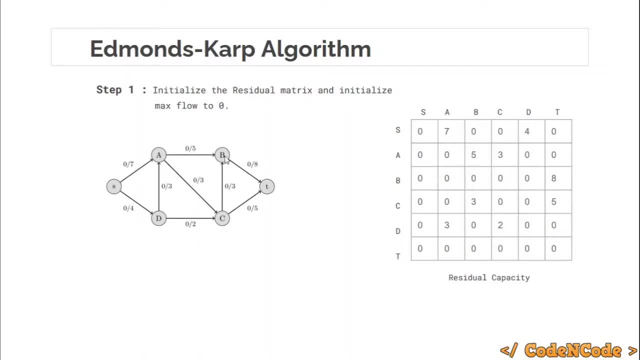 so it represents the capacity of edge, this edge from A to B. now this represents the residual capacity of the whole graph. now, as you might remember from the previous lecture, we have seen what is residue er, the residual capacity, residual graph, reverse uh Capacity. so I hope you have was a previous lecture because there are many things that you must know now, since, from s to a, the capacity. 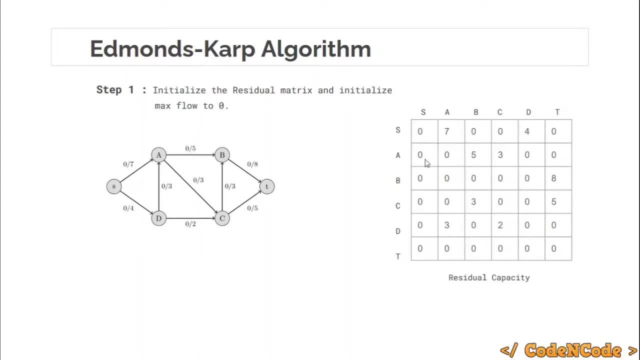 Or the residual capacity is 7. so from a to s, the capacity would be 0. A to s, you can see, the capacity is 0 because since there is no flow in the original Original edge- I mean in the edge s to a- there is no flow. 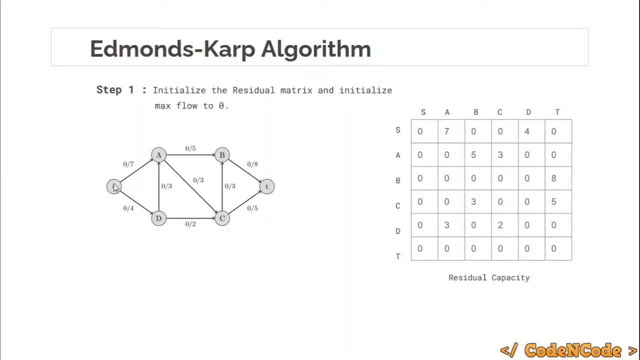 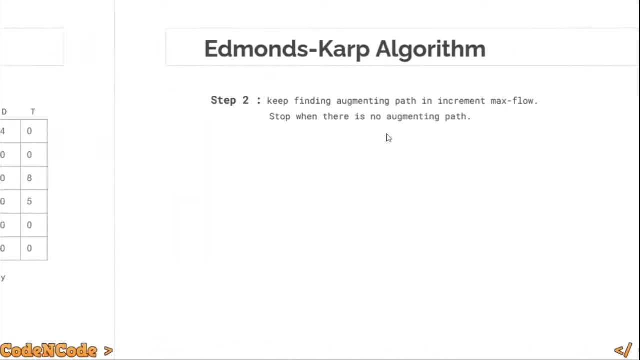 so from a to s, the reverse edge, the imaginary reverse edge, the residual capacity would be 0 because, reverse, for the reverse edge, the residual capacity is equal to the flow in the original edge. now, After step 1, step 2 is the finding the augmenting path. keep finding the augmenting path till we have one. 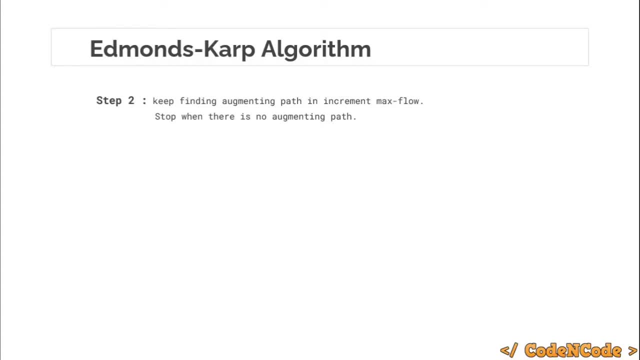 so once we do not have any augmenting path, that is where we stop and That represents your maximum flow. so, basically, you would initialize the max flow to 0 each time you you keep finding the Next augmenting path and incrementing the max flow. and how it is done. Let me explain you. 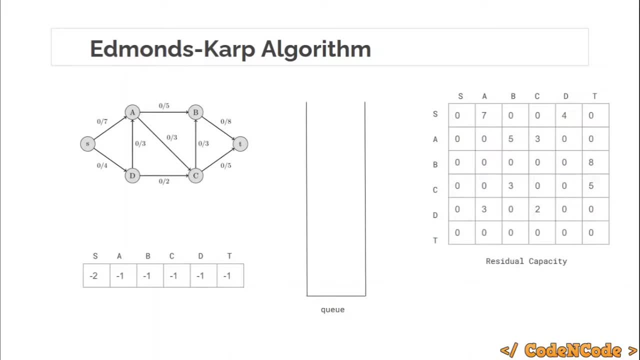 So, since we already know that admin cop uses BFS, so this is Q. There is the original graph. This is a general capacity Matrix and this represent parent of each or each node. So why do we need Keep track of the parent? is that Once you find an augmenting path, you actually need to know all of the of the nodes on the augmenting path? 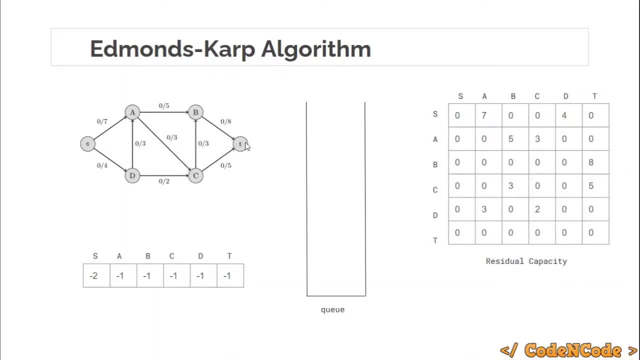 so if I found this Path, I need to have the knowledge that the path consists of s, AC&T, and this is what enables you to do it, to basically remember the path. so parent of T would represent the. this is the parent that is. minus 1 represents we haven't found any parent and minus 2 represent it doesn't have. 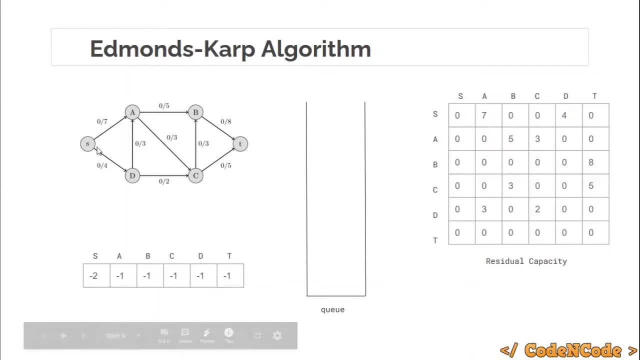 parent because source is the point where you start, so it has no parent. parent is the node from which you came to this node. for example, if the augmenting path was this: as a, B and T, then the parent of T would be B, because you came to T from. 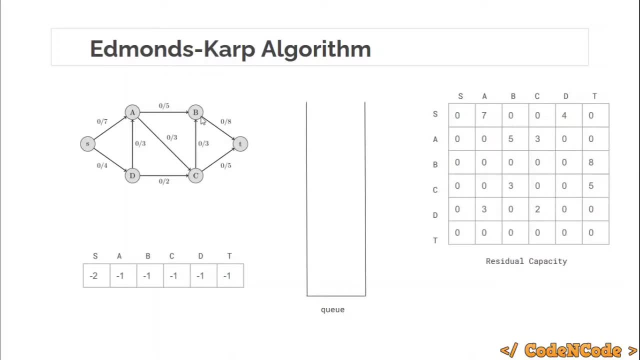 B. so parent of T would be B. similarly, for parent of B would be a. so this array here keeps track of parent of each node, since source has no parent. that is why I've initialized it with minus 2. now, if you have the knowledge of parent of each, 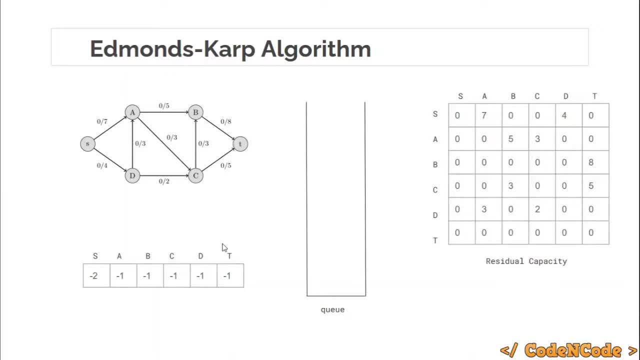 node. then you can actually find out the the path. so if parent of T is B, then you'd go to B. parent of B is A, so you would go to A. parent of A is S, so you would go to S and finally you have found the whole path. so it is T A B S or S A B. 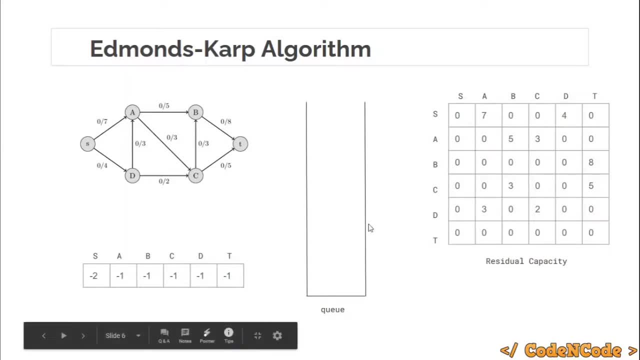 T. so that is why we are using the parent array. now. this is Q, which is the standard BFS procedure. this represents the front of Q and this represents rear of Q. basically, any deletion would take place from here, any addition would take place from this side. so now what we would do. 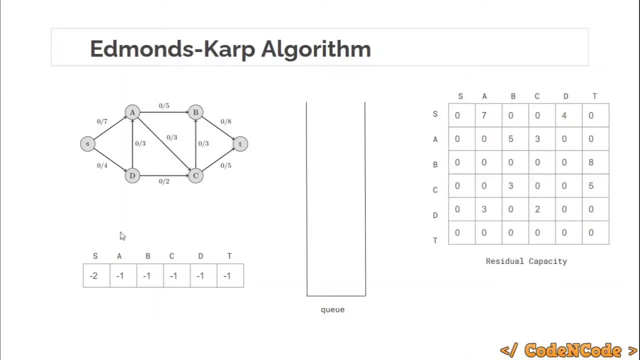 of course we will do the basic BFS stuff that we do what we do. we would insert source in it. so source with the minimum capacity found till now- infinite. now, what is this see when we are finding the augmenting path? if we find the augmenting path like this as A, B, T, the minimum capacity on this path is 5. 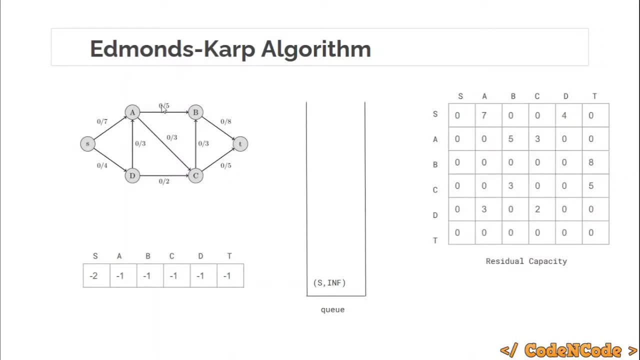 so 7, 5 and 8, so the minimum is 5. so basically, on this path you can send 5 amount of of flow and that is why you need to keep track of minimum, since we need to keep track of minimum. this, the second second parent parameters, represent: 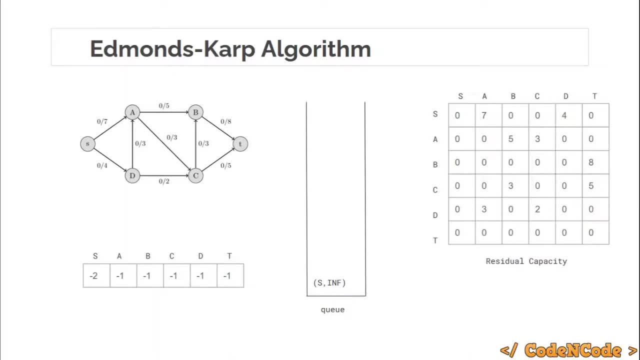 the minimum of path found till now. so, since we are just starting, so I'll be keeping this infinity. now we will take out S, because what happens now? the BFS starts. so first we see whether the queue is empty or not. of course the queue is not empty would take out the first element, which is S. so S is connected to 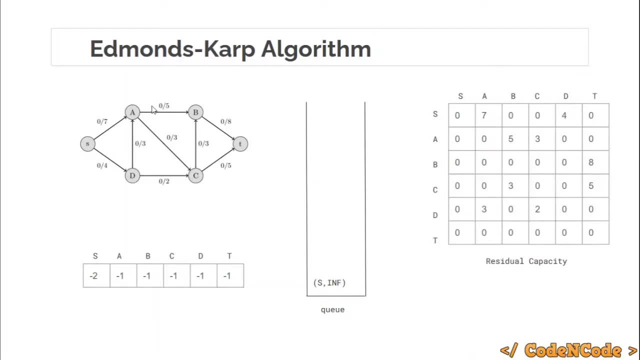 A and D. right, so we would insert A and D, both now S to A. the minimum capacity found till now. the starting point is S and till now we have reached A, so minimum capacity found to this path is 7, so that is why we are having 7 here. 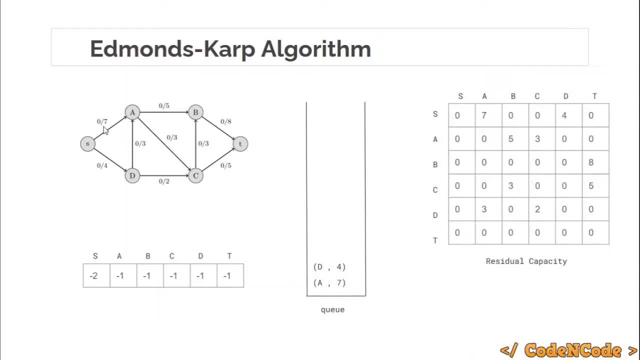 basically minimum of parent comma, the new edge. so infinity comma 7 is 7 and for 4 it is infinity comma. minimum of infinity comma 4 is 4. so on this path, minimum capacity found till now is 7. on this path, minimum capacity found till now is 7. on this path, minimum capacity. 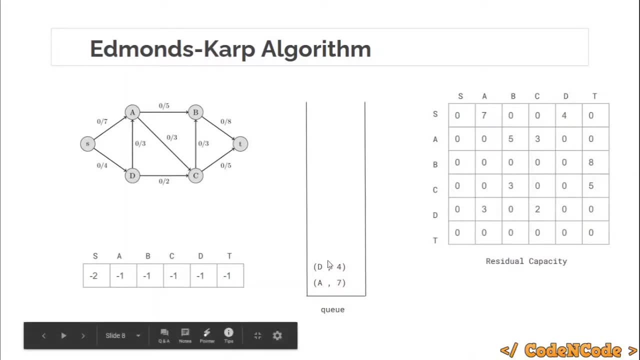 found till now is 4, so we have inserted D and A both with proper minimum capacities and now in the parent array, since you have reached D and A from S, so parent of D and A would be S, so parent of D and parent of A is 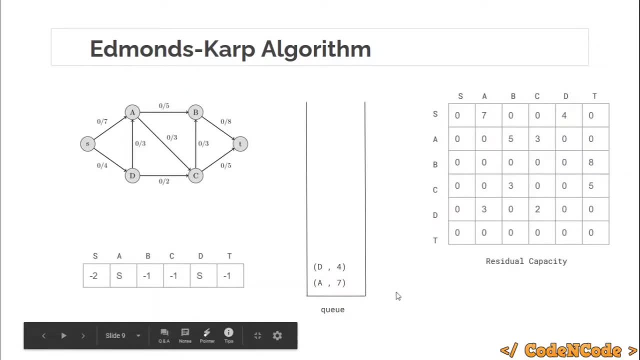 updated to S. now again you see whether the queue is empty or not. of course the queue is not empty. so you take the first element out, which is A, comma 7, and then you see that what are the nodes which are: A connected to A is connected to B, C, 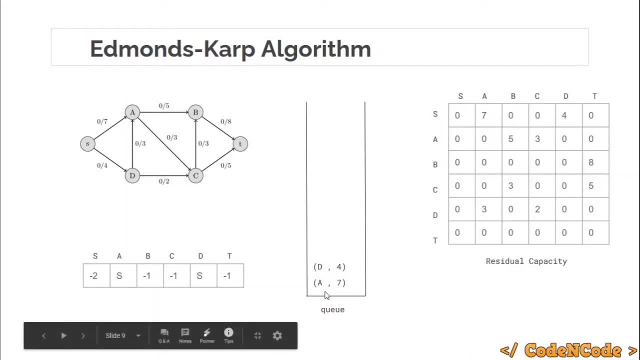 because we are taking out first, which is A, comma 7, so A is the next node we are working with, so it is connected to S, D, C and B. yeah, one more thing: when working with admin curves, you would assume that the graph is actually undirected reason. 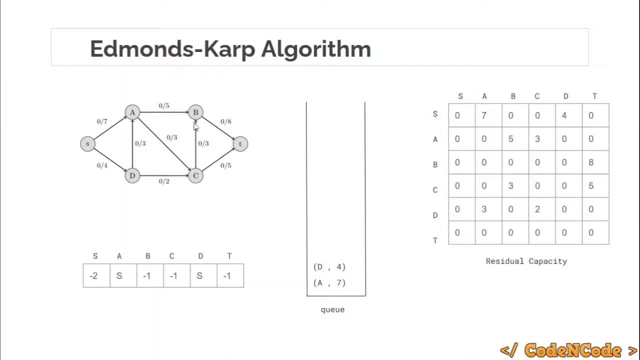 of course, because we have both the edges. if you have one edge, we have both the edges, because we are assuming there is an imaginary reverse edge and that is why we are considering it as undirected graph. so s is connected to s, d, c and b. but the problem with s and d is that they are already visited. how do we know? 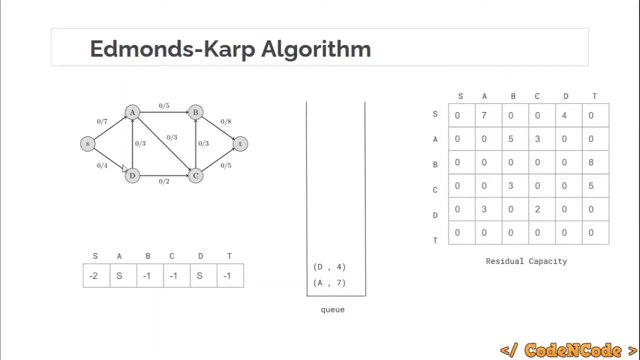 that if they are not visited then their parent would be minus one, but parent of s is not minus one, parent of d is not minus one. so these two are out of option. we are left with b and c. so we will insert b and c because b and c are not visited yet. so from a we would 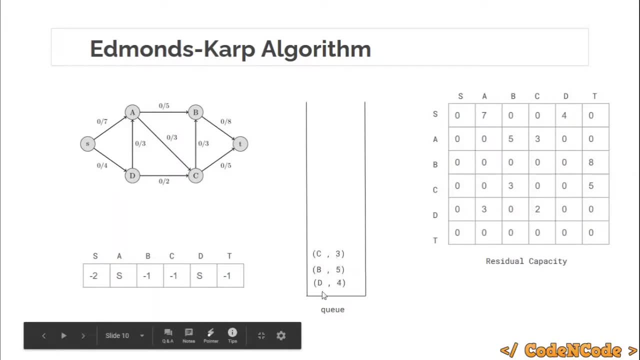 insert b and c. so i have inserted b and c and removed a comma seven. now it was a comma seven, so minimum was seven till now. so the minimum till b would be minimum of seven comma five. minimum of seven comma five is five, so of course it is five. for c it would be minimum. 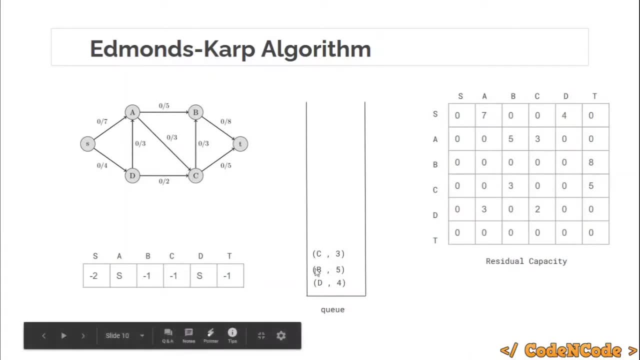 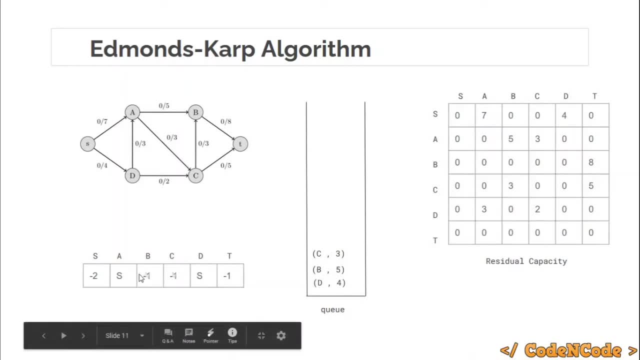 b and c. we need to update their parents at the as well. parent of b and c would be a. now we take out d, since d is connected to a, c and s. the problem is all of them are visited, so d cannot add anything, so we'll simply remove d. now it's time for b from b. b is connected. 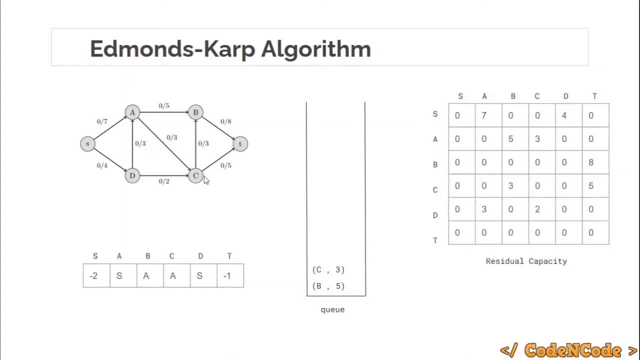 to a, c and t. while a and c are already visited, we have only left with one option: to insert b. so we insert t, comma five, because till b it was how much it was t till t, sorry, till b it was a five minimum, till b was five. now minimum. till t would be minimum of five comma. 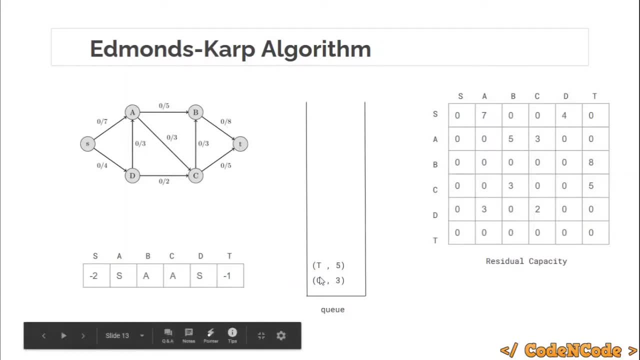 eight, which is five, of course. so t five is added. now, since we have added t, we need to update the parent of t, which is b, because we have k, because t is traversed from b. so parent of t is equal to b. now, as soon as you reach t, you know that you have found an augmenting path. 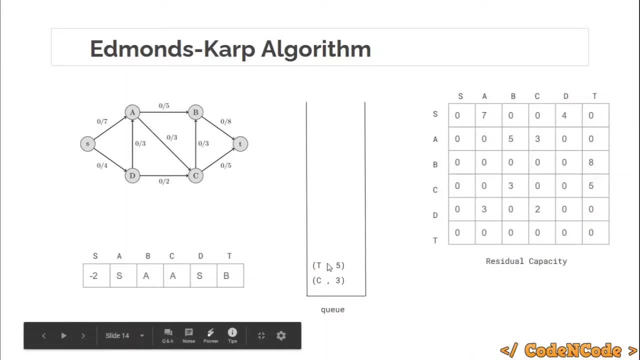 because we have started from s. now we are at t now, since we have found a augmenting path which is having minimum capacity, uh, the augmenting path is having minimum capacity five, so we will return five, indicating that we can increment. we have found, uh, an augmenting path which is having 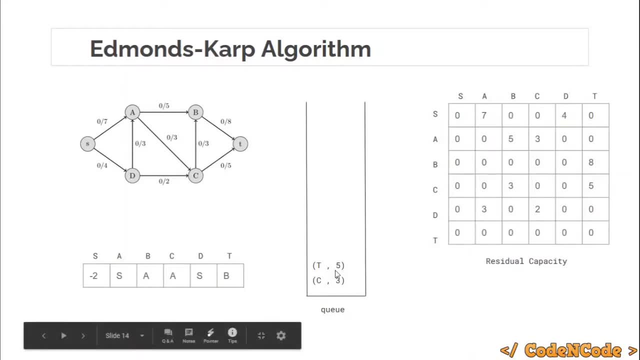 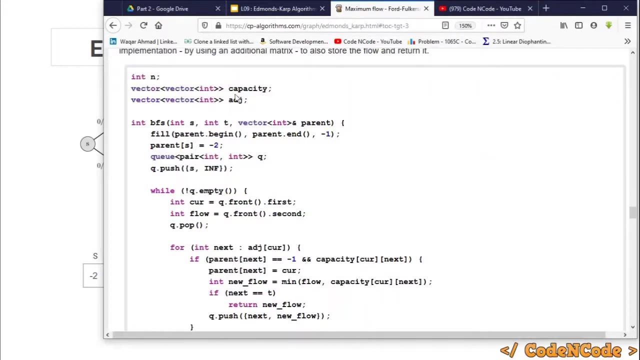 the minimum capacity: five, so we can increment or send a flow of value five. so, basically, we are going to increment the flow five, uh, by five. so let me show you the algorithm how it works. so here you see. uh, this is a 2d grid to represent the residual. 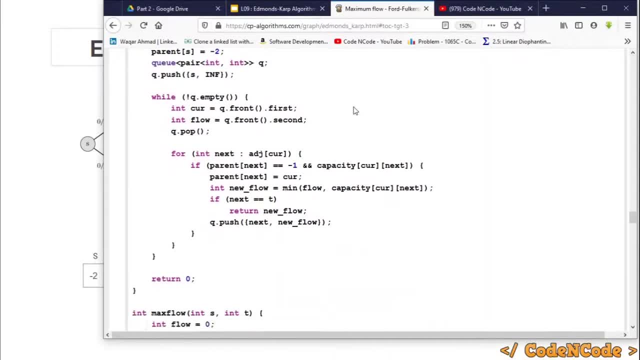 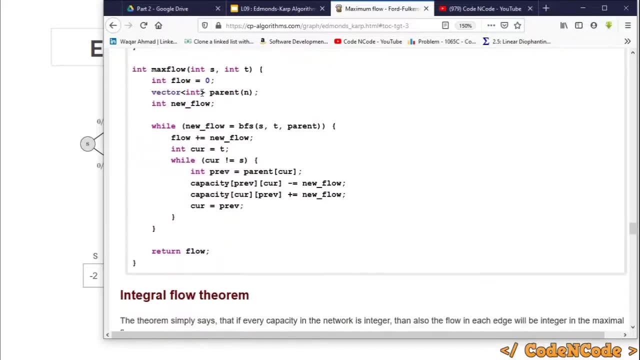 capacity and this is the adjacency list. now, what is happening here? see, we are in. this would return the maximum flow, and this is the bfs- bfs part. so what is happening here? flow is initialized with zero and here we are finding the flow and finally returning the maximum flow. now what? what? here we are doing. 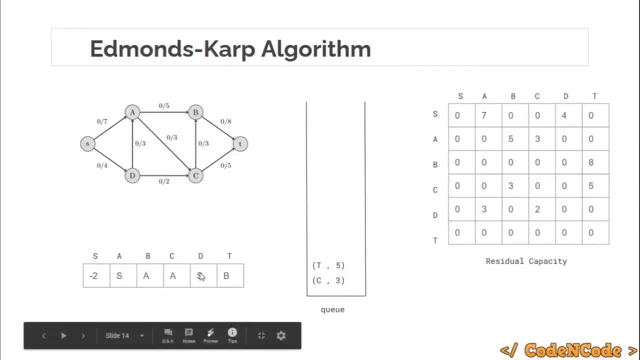 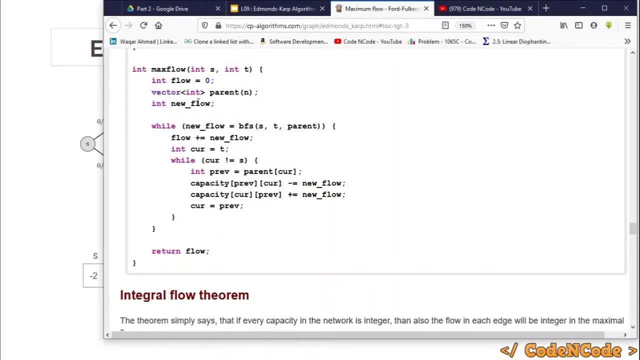 we are initializing the parent array, this array. now we are initializing the parent array. uh, basically, yeah, initializing the parent array and new flow. we are also using new flow variable now, while new flow is equals to bfs of s, t and parent, we are passing the parent array. 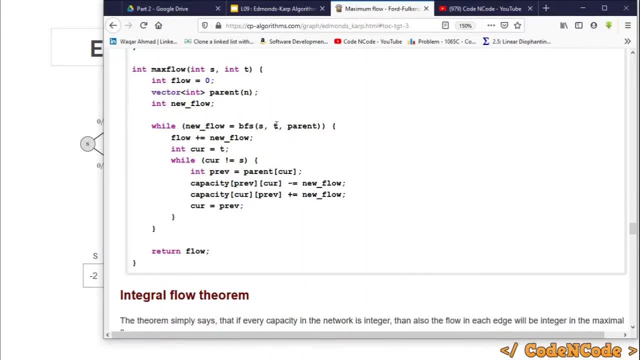 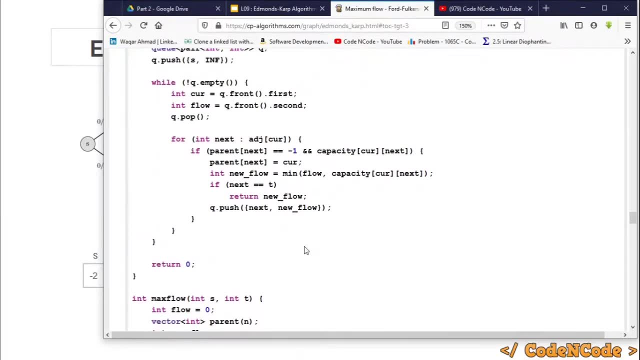 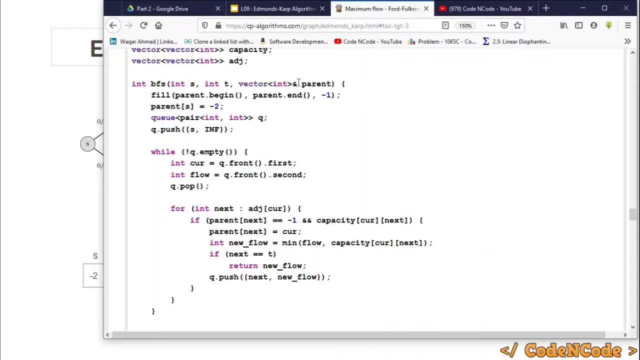 source and time rating point. now, bfs would return the maximum flow augment maximum, basically minimum capacity of augmenting path, if it finds one. so what it does? it receives three parameter, of course, and make sure that you pass parent array using reference, otherwise you may receive tle. now we are filling the parent array. 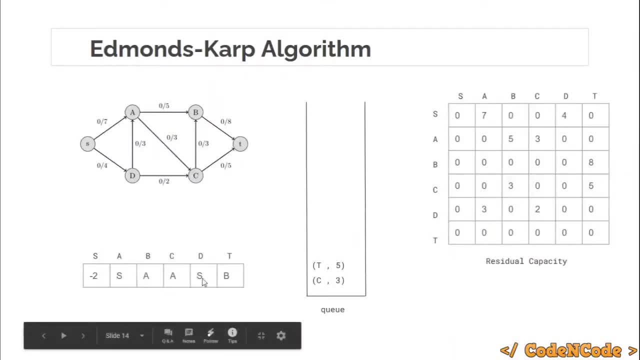 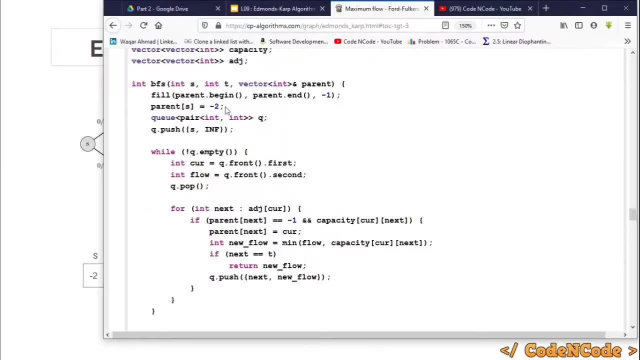 with minus one, as i have done. initially, all of the values were minus one in uh, only for source it was minus two. so for source- parent of source- we are starting with minus two now. this is just to store the, the pairs, in the queue and we are inserting the q- source comma, infinity, the step one and then. 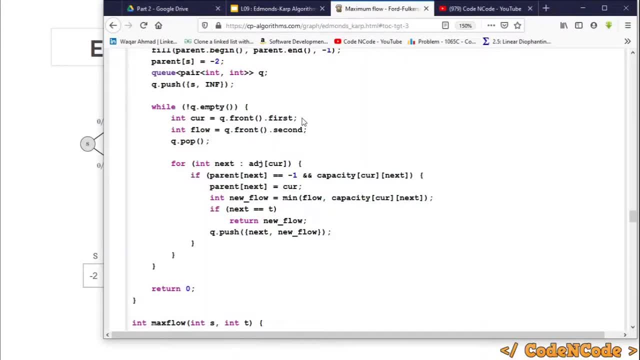 the usual bfs system, you take out the front and current node is q dot front dot. first, because first represents the node. second represents the minimum uh, minimum capacity found till now and the flow is equals to q dot front dot. second, and you, of course, remove that. no uh, remove that. 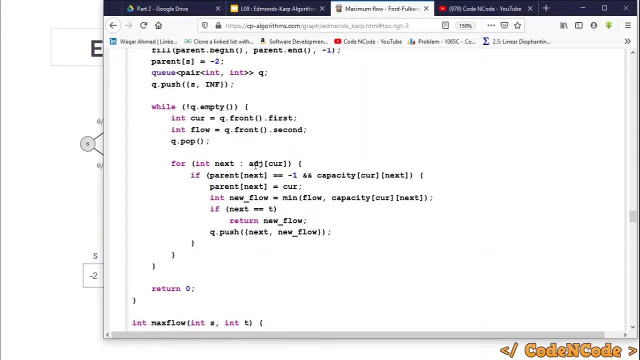 pair from the queue and for each node in the adjacency list of current node what we would do. you would see whether its parent is equals to minus one. if its parent is equals to minus one and the capacity, the residual capacity, is positive, so it is checking for the residual. 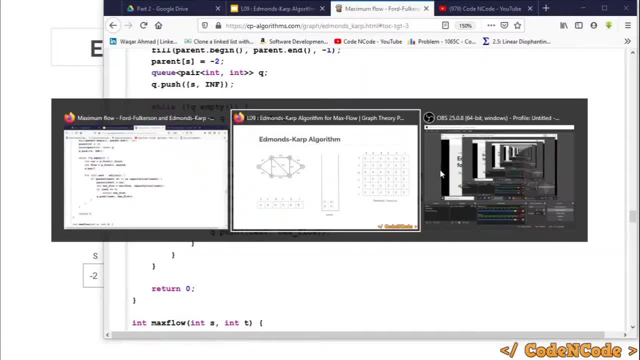 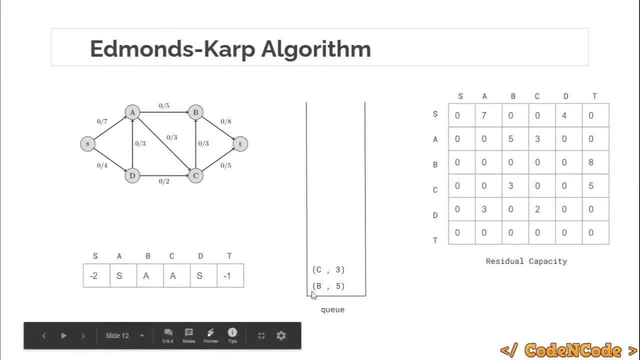 capacity to be positive if both the condition are true, basically you. for example, if i go back here, if i take out b in the adjacency list of b, i have c, a and t, but a parent of c is not minus one, parent of a is not minus one, but parent of t is minus one, as 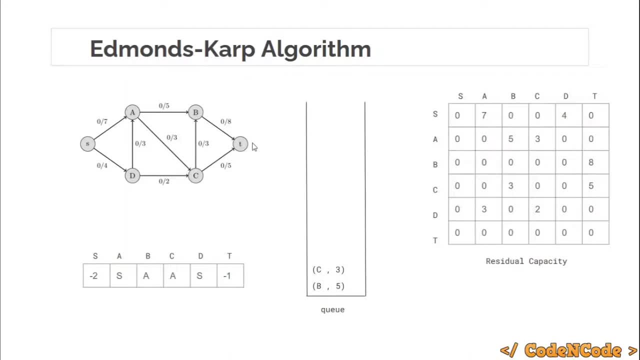 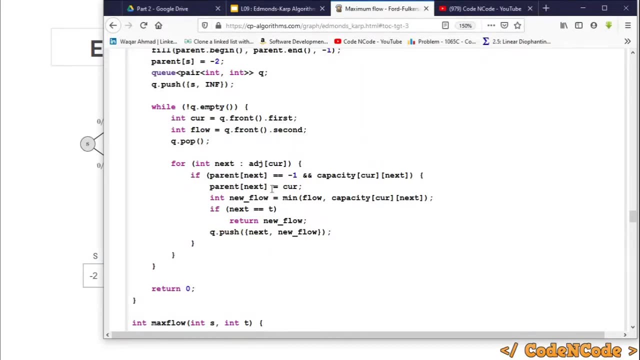 you can see. so i can go to t and residual capacity of b comma. t is actually positive. that is why i can actually insert it into the queue. so first i will be setting the parent of it and then we will be calculating. the new flow would be the flow found till now. comma. 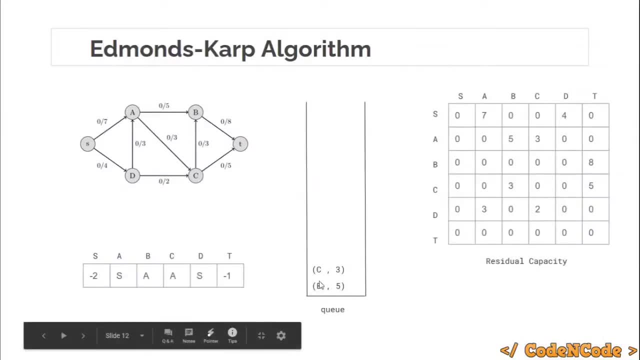 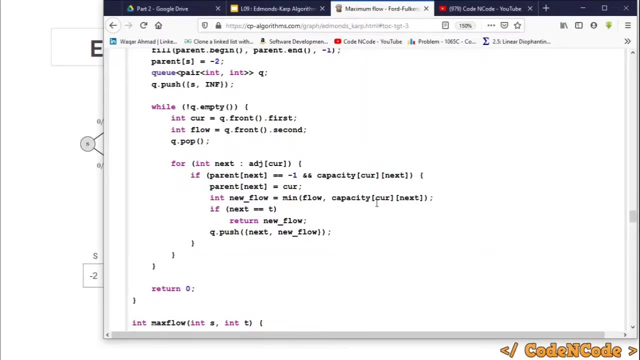 the new capacity. basically, you are calculating the minimum of b comma t, right? so new flow would be: uh, the minimum of flow found till now. comma, the. uh, the residual capacity of the edge, current comma. next, if you have found, if the next node is actually terminating point, then we are going to. 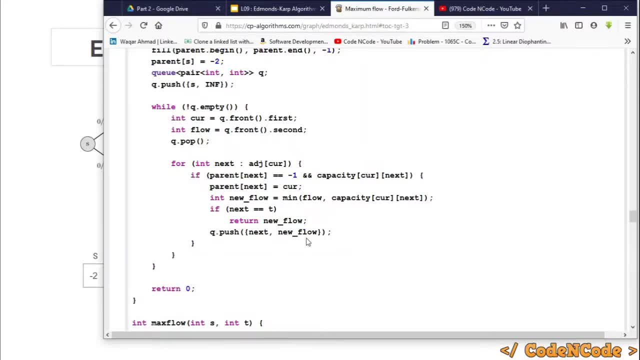 return the new flow, otherwise we are going to insert it into the queue. if, after running this while loop, we haven't found any augmenting path, if you haven't found any argument in path, this line won't be executed. basically you'll end up here. if you end up here, basically you have not found any augmenting path, and that means your. 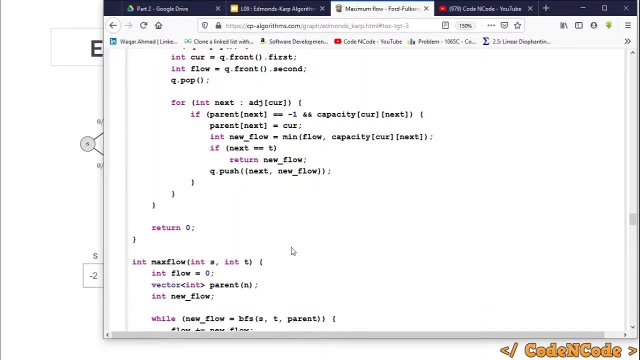 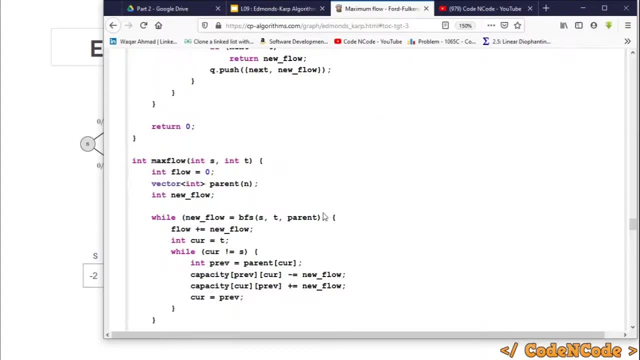 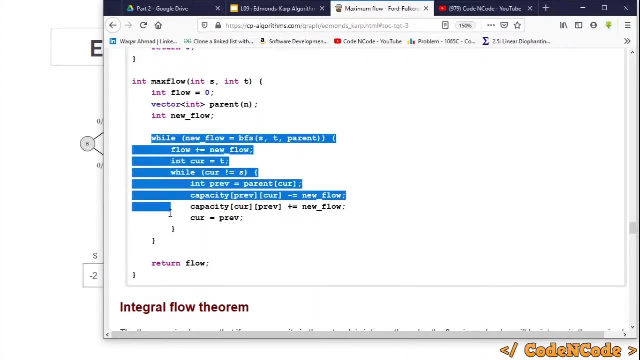 graph doesn't contain any augmenting path. if your graph doesn't contain any augmenting path, you would return zero. so that explains this while condition. so if bfs returns zero, so a new flow would be zero. if in the condition you have passed zero, you would basically terminate. so if you have found no argumenting path, it would return zero. 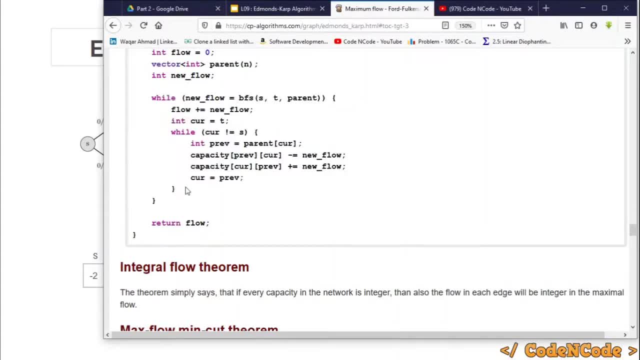 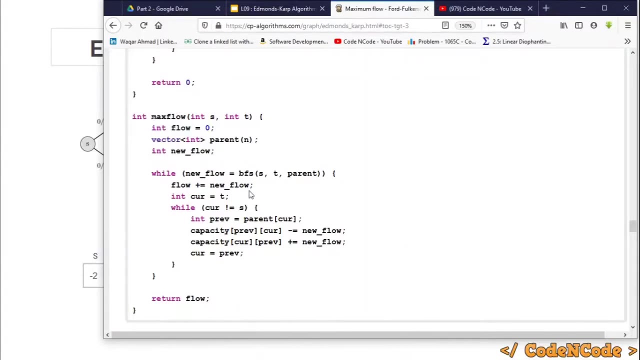 and if it returns zero, this while loop will stop. so basically, we are stopping when we don't find any augmenting path. otherwise it returns the new flow. if you have found the new flow, what you would do? you would uh, in the flow, you would add the newfound flow, and then we need to update the 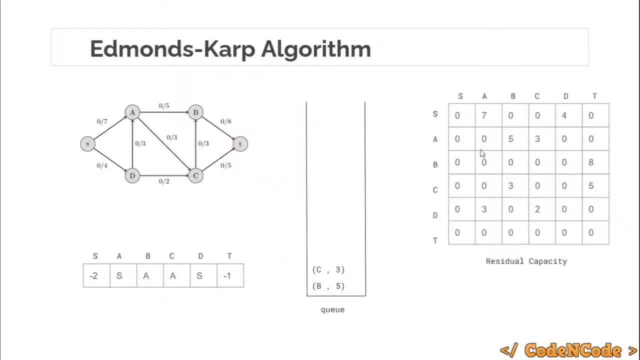 residual graph. let me show you how the residual graph is updated. so let's go and update, update the residual capacity graph. so what would happen? uh, to update it, we need to find the path, augmenting path. and since we have found this augmenting path, which is uh, which uh, 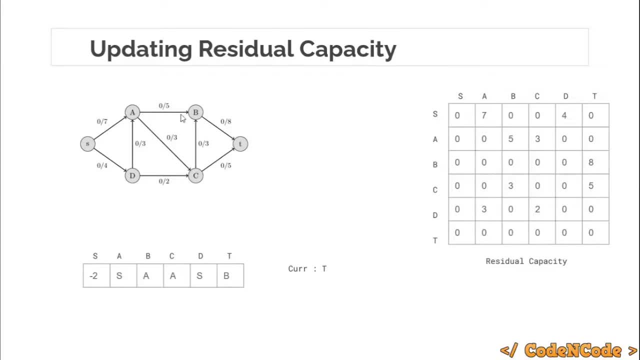 using which we can increment the flow by five. so basically, we need to reduce the capacity of this path by five and also increment the flow through these edges by five, right? so initially, the current node is going to be terminating point. so parent of t is b, so we are talking about the. 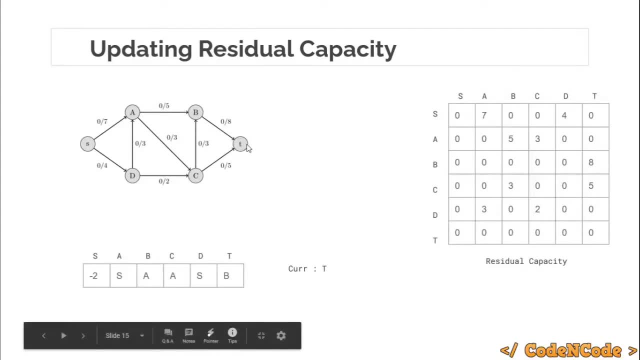 edge bt right. so the the capacity, the residual capacity of bt would be reduced by five. so bt would be reduced by five. so i have reduced bt by five. and one more thing: since you have reduced the capacity of residual capacity of hbt by five, you would increment uh. now you would. 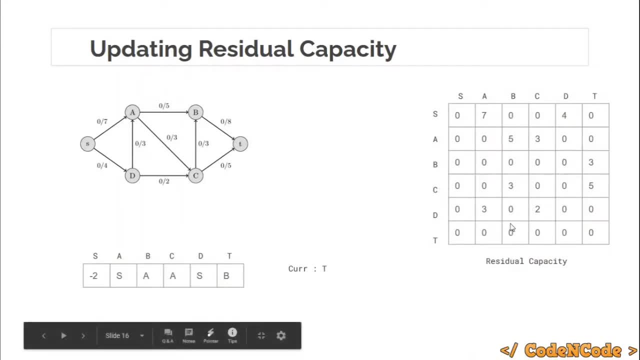 increment tb by five as well. i have not shown it here because it represents the reverse edge, because bt is the original s, so tb is actually reverse edge. so, uh, since there is now a flow from bt of value five, if you remember from the previous lecture, if there is a flow f in the 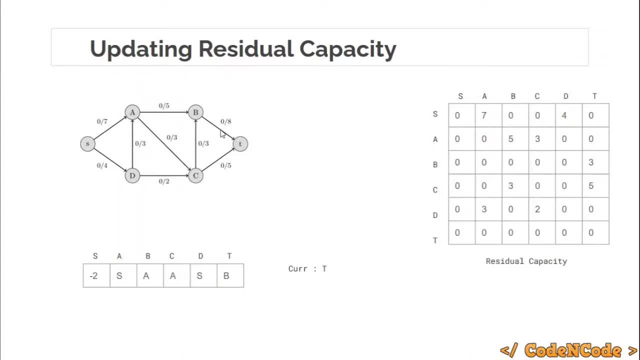 original graph. then the residual capacity of the reverse uh reverse edge would be plus f as well. so since you are reducing the capacity of hbt, you would increment in tb. so this would be plus five zero plus five uh. i haven't shown that about the reverse edge and that you can found. uh, you can see. 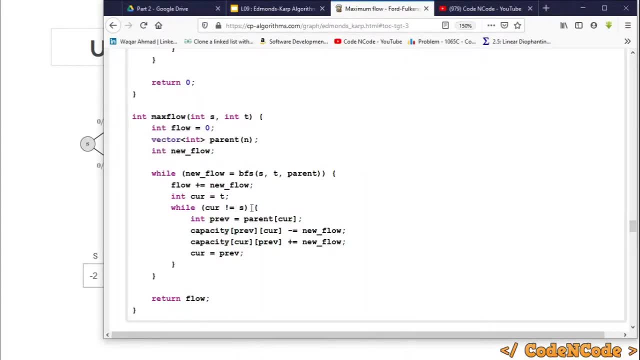 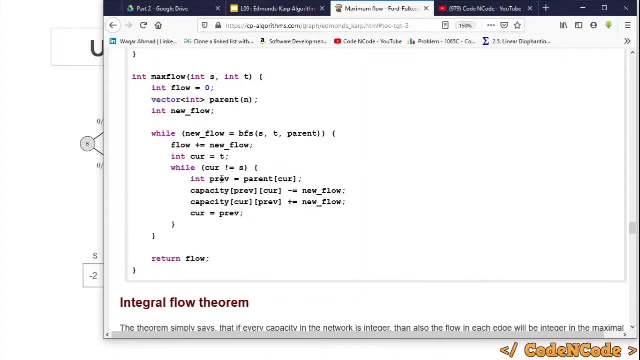 here. so current is equals to t, basically your terminating point. while current is not equal to s because s does not have it. so current is not equal to s because s does not have it. so current is not equal to s because s does not have it. any parent. so while current is not equal to, at what you do, you would find the parent of it, which 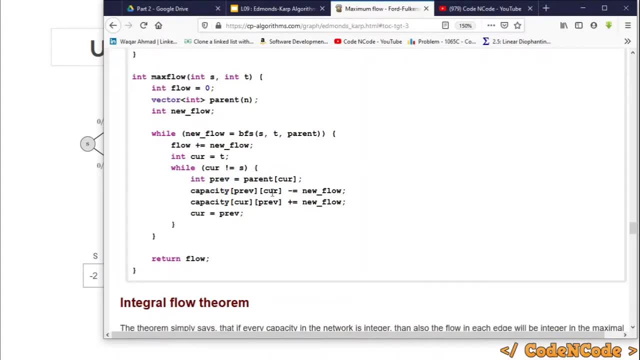 is called previous here, and the capacity of previous comma, current, would be decremented by flow and capacity of a current comma, previous- basically, the reverse edge- would be incremented by the new flow and, of course, current is equals to previous, so current was it. now current would become. 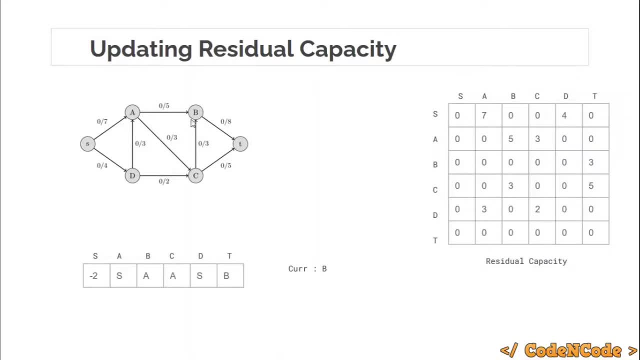 b, because now we have taken care of this edge, now i'm here and i'll be taking care of this edge how now. current is equals to b, the parent of b is equal to a, so now i need to reduce the uh residual capacity of edge a b. so what i would be doing in the a b cell, i'd be reducing it by five, so it